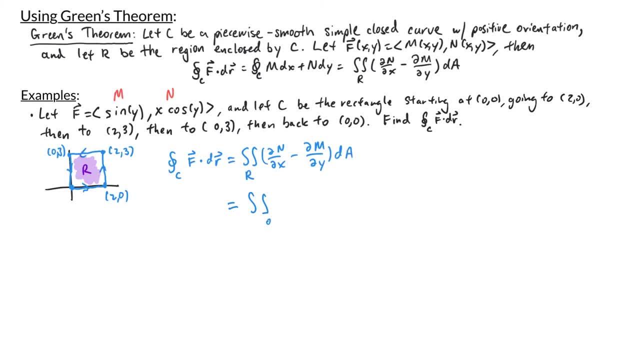 dx. So my first limit of integration would be from 0 to 3 and then my second limit of integration would be from 0 to 2.. Now partial derivative of n with respect to x would be cosine of y, and I subtract the partial derivative of m with respect to y, That's going to be cosine of y. 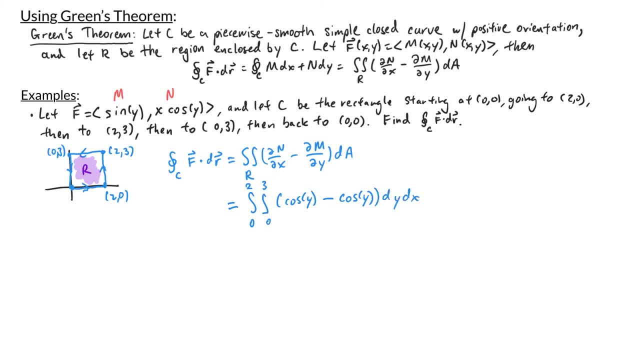 again dy, dx, and so this is just the integral from 0 to 3, from 0 to 2, of 0,, dy and dx, and that gives us 0.. Now this answer should make sense to us, because here the partial derivative of n with 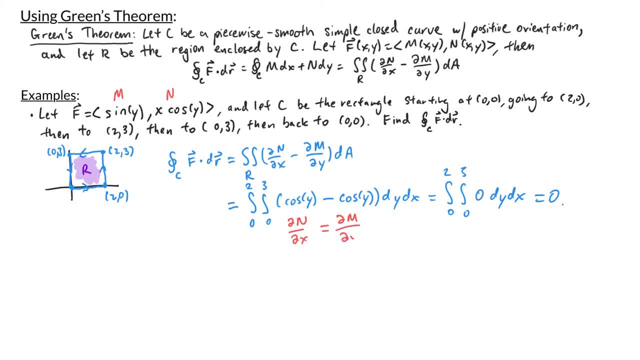 to x is the same as the partial derivative of m with respect to y, which tells me that f is conservative And for conservative vector fields the line integral over a closed curve is always zero. Let's consider this next example. So we're asked to calculate the line integral of 3y. 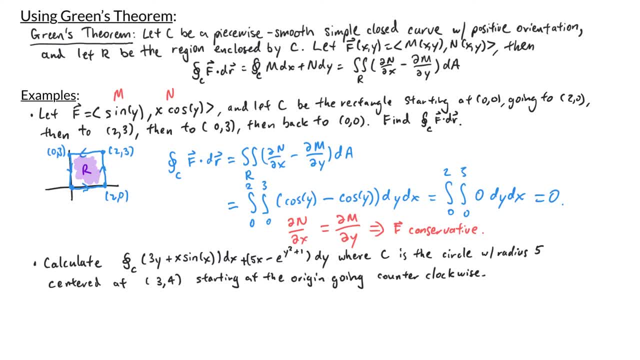 plus x sine x, dx plus 5x minus e, to the y square plus 1 dy, where c is the circle with radius 5 centered at, starting at the origin and going counterclockwise. Let's start by drawing a quick picture. We have a circle centered at, with radius 5,. 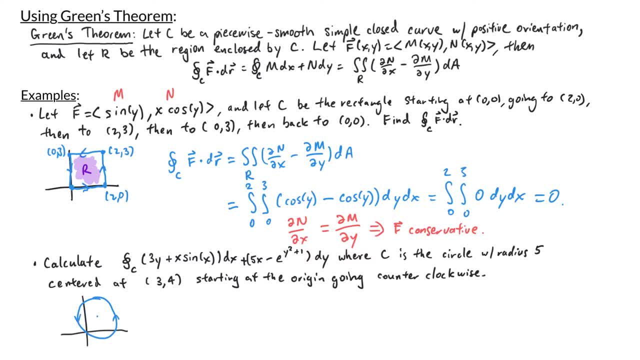 so maybe something that looks like this, going counterclockwise. So while this line integral isn't written in the form f dot dr, we can think of it that way by taking f to be the vector field, with x component, 3y plus x, sine x and y component. 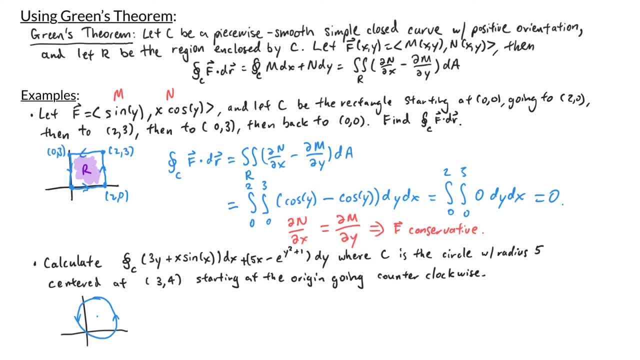 5x minus e to the y square plus 1.. So here m is 3y plus x sine x, and n is 5x minus e to the y square plus 1.. According to Green's theorem, the line integral of m, dx plus n, dy is the double integral over. 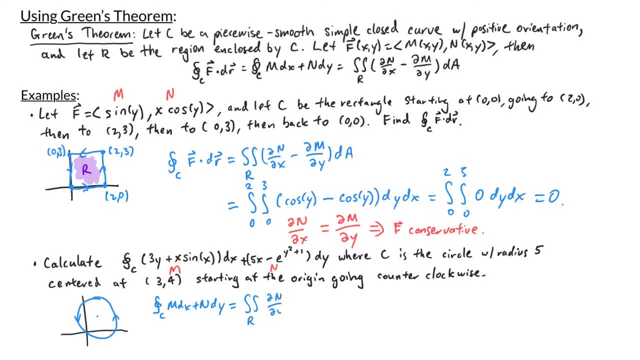 the region R of partial derivative of n with respect to x, minus partial derivative of m with respect to y. da r is the region inside the circle. So here we have the double integral over the region R of the partial derivative of n with respect to x. 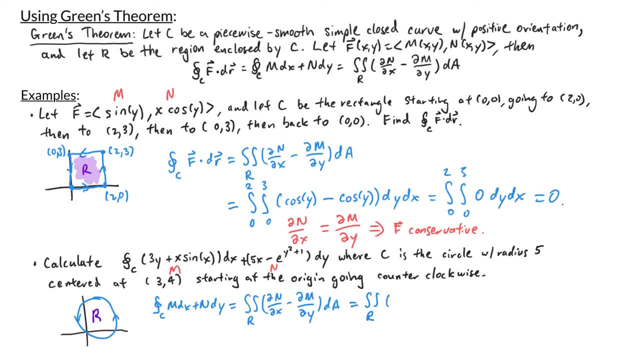 Since n is 5x minus e to the y square plus 1, this partial derivative is just 5.. Then I have minus partial derivative of m with respect to y. m is 3y plus x sine x, so the partial derivative is just 3, da. 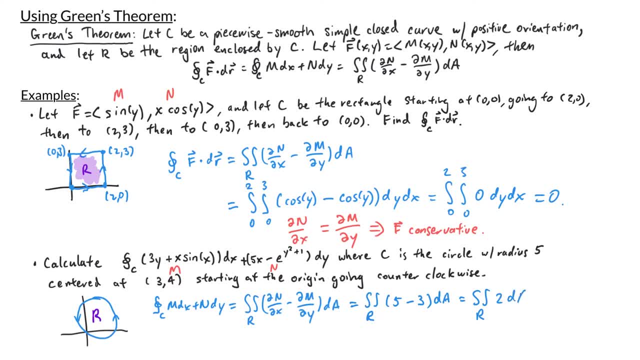 So I'm looking at the double integral over the region R. I'm making a double integral of 1, da. So I've just taken a double integral for the region R of 2, da. If I factor the 2 out, this becomes 2 times the double integral over the region R of 1,. 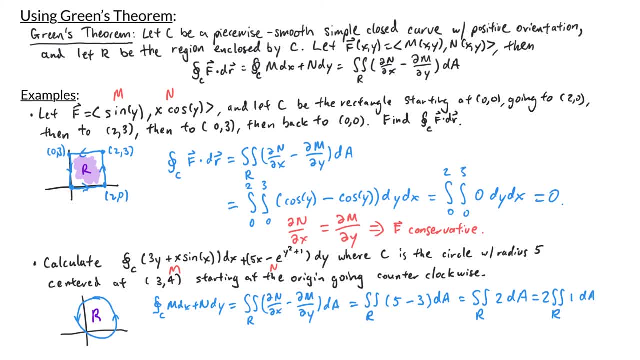 da. Now, if you recall, whenever I have the double integral of 1, da over a region R, that's just the area of the region R. So this is 2 times the area of R. Well, R is the circle with radius 4.. 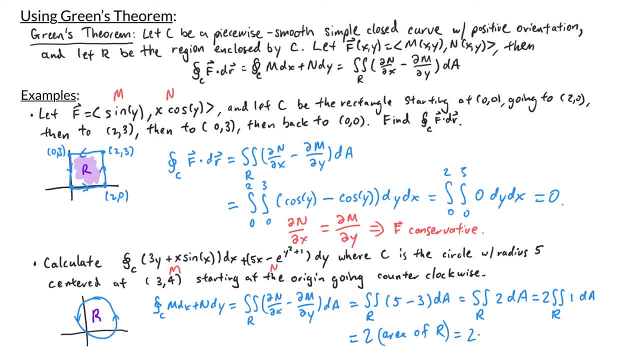 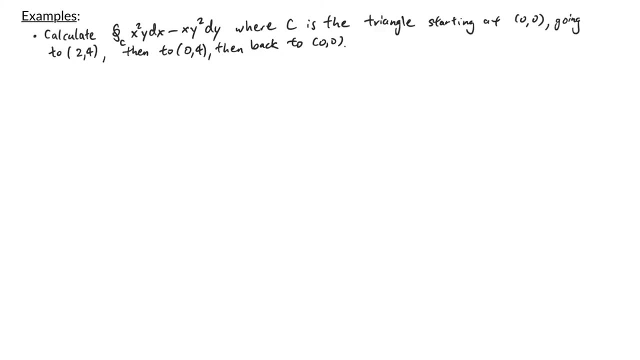 This is R, This is R, So this is r 5. so its area is pi times 5 squared. so this simplifies to 50 pi. Let's look at a couple more examples. In this example we're asked to calculate the line integral of x squared y, dx minus x, y squared dy over the curve c. 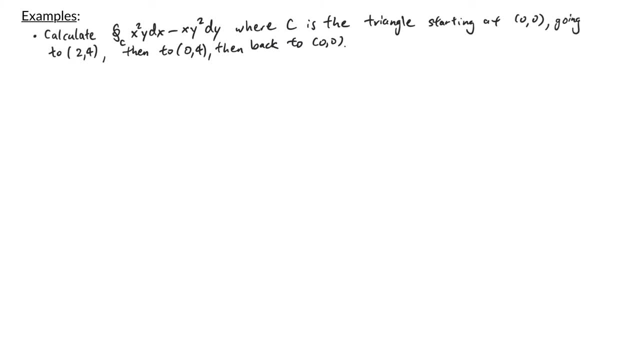 where c is the triangle starting at the point zero, zero going to two four, then to zero, four, then back to the origin. As always, I'll start by drawing a picture of this curve. So I have the curve starting at zero, zero going up to two, four, going over to zero, four. 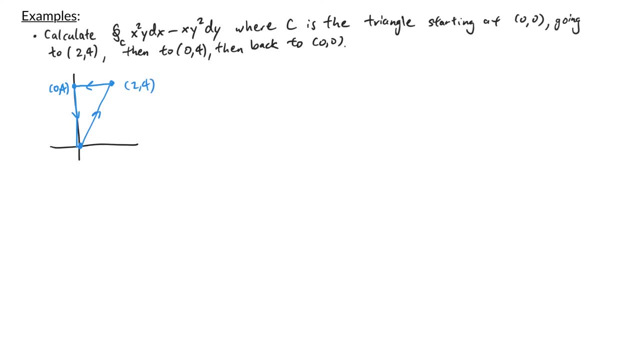 and then back to the origin Again. Green's theorem tells me that the line integral of m, dx plus n, dy is the double integral over the region r enclosed by our curve of partial derivative of n with respect to x, minus partial derivative of m with respect to y dA. So in our case m is x squared y. 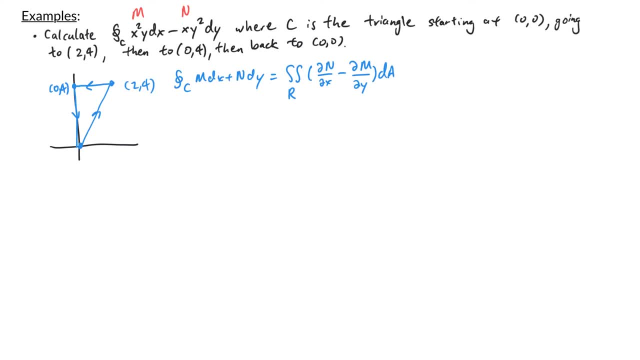 and n is negative, xy squared. Now here, my region is this triangular region, and when I'm doing the double integral, I have a choice of doing this with respect to y first, then x, or x first then y. Let's choose to do this with respect to y first, So my bounds for my y the lower. 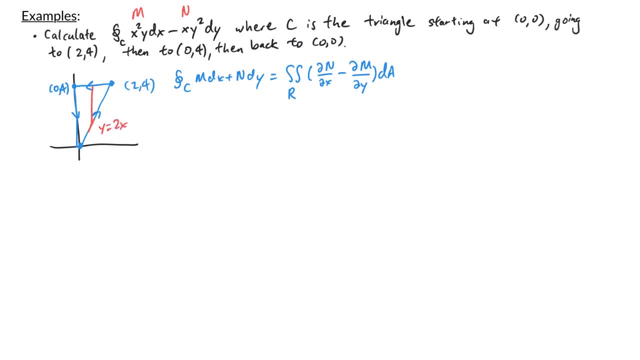 bound would be the line y equals 2x and the upper bound is y equals 4.. And in this triangular region my x's go from 0 to 2.. So we have the double integral of the partial derivative of n with respect to x. n is negative, xy squared, so its partial derivative with: 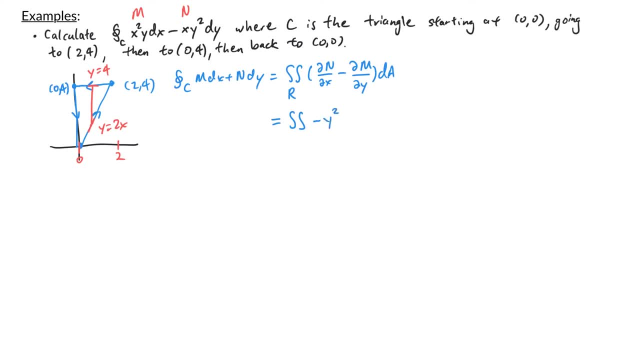 respect to x is minus y, squared minus the partial derivative of m. with respect to y, m is x squared y, so my partial derivative gives me x squared. here And again I'm doing my double integral in the order dy- dx, where my limits for the y 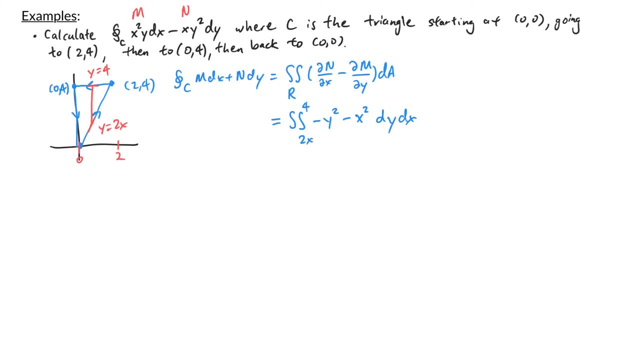 are 2x to 4 and my limits for the x are 0 to 2.. I won't go through the details of this calculation, but you should end up with negative 104 over 3.. I want to mention that doing the line integral. 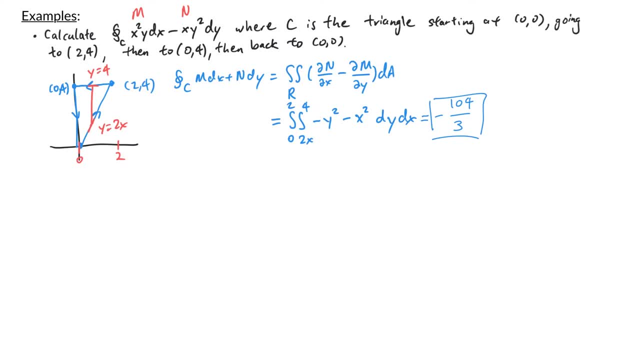 without Green's theorem would be much more tedious. You would need to break apart the triangle into three different segments, find parameterizations for each of those segments and then evaluate the line integral on each segment. So Green's theorem is a really useful tool in helping us compute the line integral. 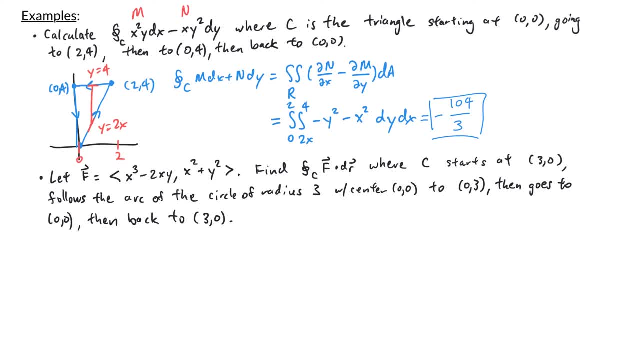 Let's look at one last example. Here we have the vector field f with components x cubed minus 2xy and x squared plus y squared. We're asked to find the line integral of f dot dr over a curve c where c starts at, follows the arc of the circle with radius 3 centered at. 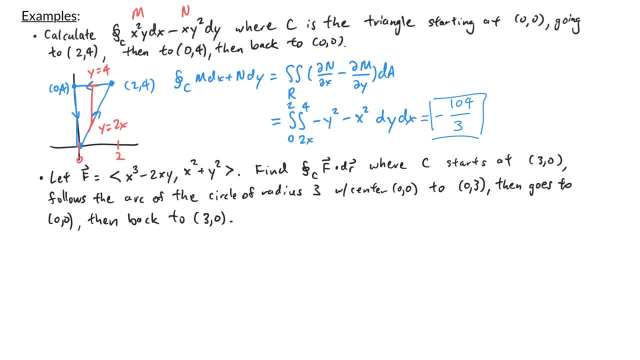 the origin to the point, then goes to, then back to. Let's start by drawing a picture: We start at and then we're following the arc of a circle to, then we go down to and then back over to. So Green's theorem tells me that the line integral. 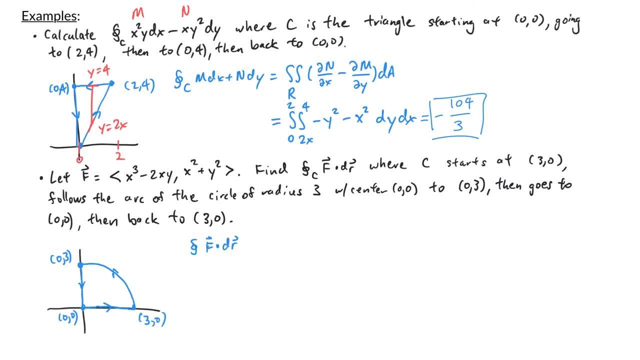 of f dot dr over the closed curve. c is equal to the double integral over the region r, of partial of n with respect to x, minus partial of m with respect to y, dA. This time r looks like a polar region, so I'm going to do this double integral.